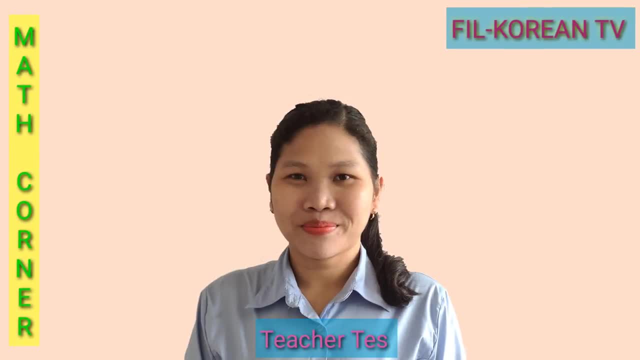 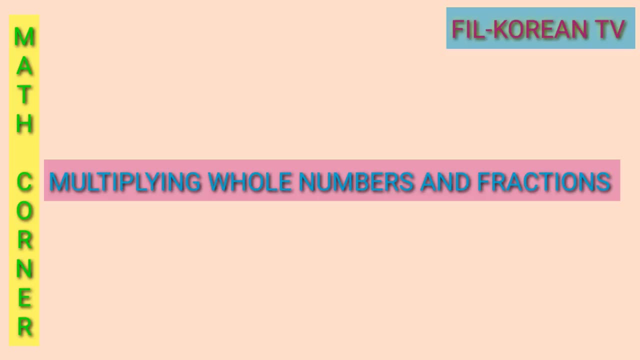 Hi, welcome to Feel Korean TV Math Corner. In this video I will show to you how to multiply whole numbers and fractions. Let's take this problem to show the step-by-step process in multiplying fractions and whole number. Okay, so let's answer 5 eighths times 2.. 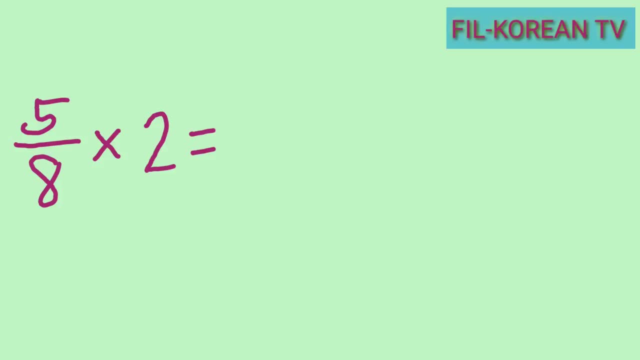 The first step that we are going to do is to change the whole number into improper fraction. We will use 1 as a denominator. Okay, let's do it. So let's write the multiplicand 5 eighths times: Okay, the whole number 2 will become 2 over 1.. 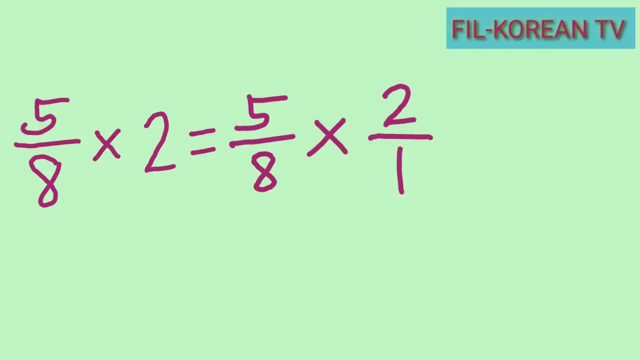 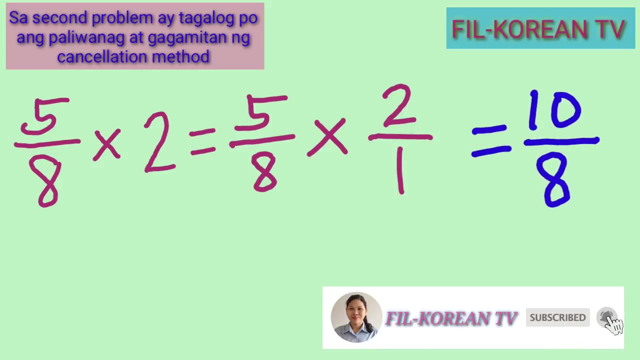 The whole number. 2 is the numerator and we use 1 as a denominator, So it is now an improper fraction. Next step: multiply the numerators and multiply also the denominators. Okay, let's multiply: 5 times 2 equals 10, and 8 times 1 equals 8.. 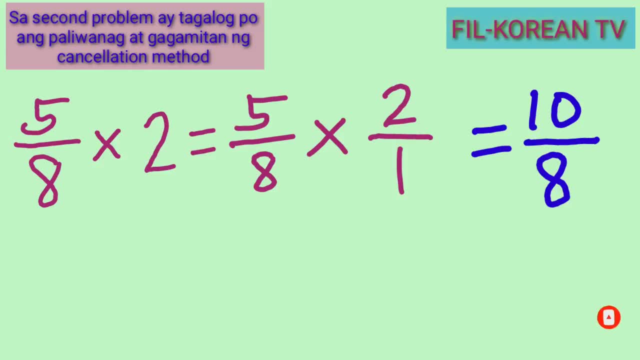 So the answer is 10 eighths. It is an improper fraction. The numerator 10 is greater than the denominator 8. So we need to simplify it by dividing the numerator by the denominator. Okay, let's divide 10 divided by 8.. 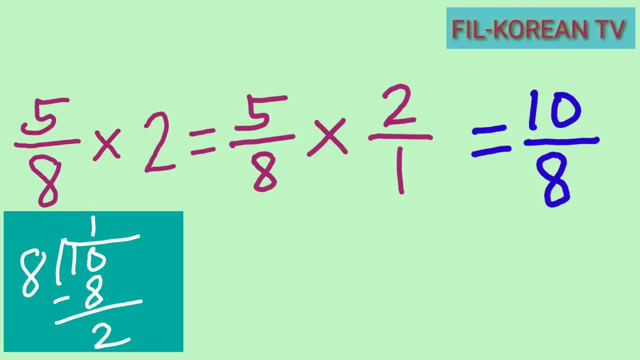 If we divide 10, divided by 8, the answer is 1 and the remainder is 2.. So the answer is 1 and 2 eighths. The quotient 1 is the whole number and the remainder 2 is the denominator. 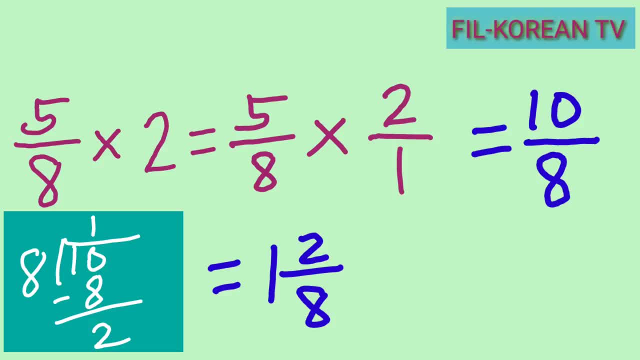 The divisor 8 is the denominator. Now look at the fraction 2- eighths. We can still reduce this to lowest term, because 2 and 8 can be divided by 2. So we will divide them by 2.. 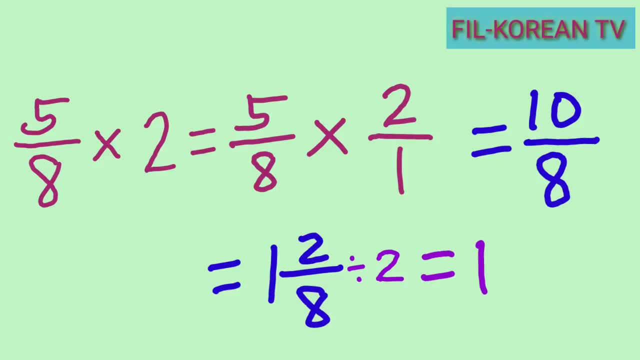 Okay, let's answer. Write the whole number 1 and then divide the numerator 2: divided by 2 equals 1.. Divide the denominator 8: divided by 2 equals 4.. The answer is 1 and 1 fourth. 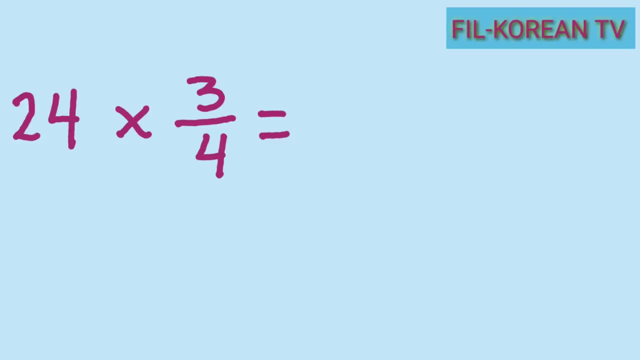 Okay, let's answer another problem: 24 times 3, fourths- Okay, so the first thing we will do is to do the improper fraction of the whole number. We will use the denominator as 1.. Okay, so the denominator 8 divided by 2 equals 1.. 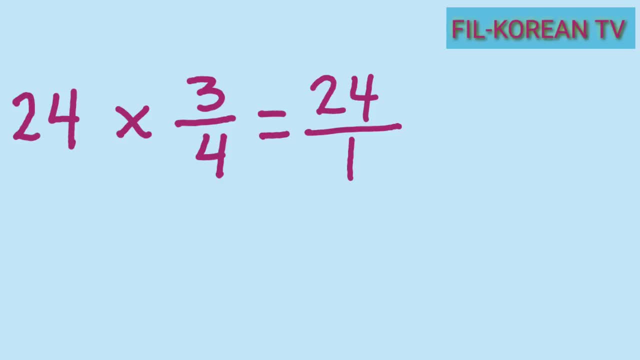 So the denominator 8 divided by 2 equals 4.. So 24 times 4 is 24 over 1.. Okay, then write the 3 fourths multiplier. For the next step: multiply the two numerators and multiply the denominator as well. 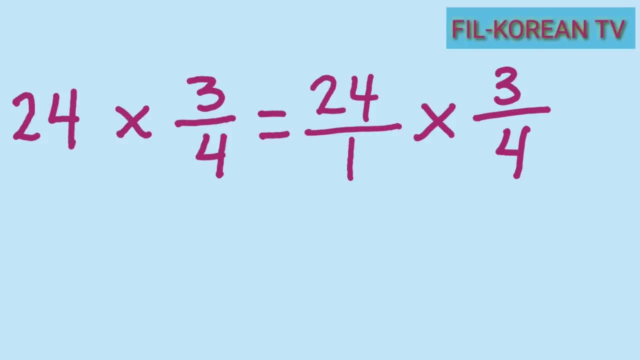 But we can use the could-be-cancellation method before multiplying to get lower the number. Okay, let's look at the numerator of the multiplicand and denominator of the multiplier. 24 and 4 have common factors, So we will divide them by their GCF. 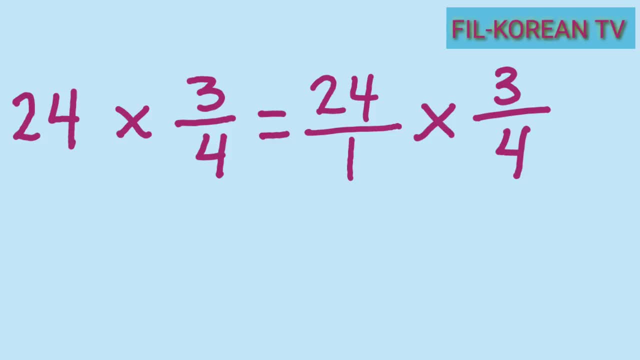 The GCF of 24 and 4 is 4.. Okay, let's divide it. 24 divided by 4 equals 6.. And 4 divided by 4 equals 1.. Yung 1 and 3 ay wala namang ibang common factor maliban sa 1, kaya hindi na natin sila. i-de-divide. 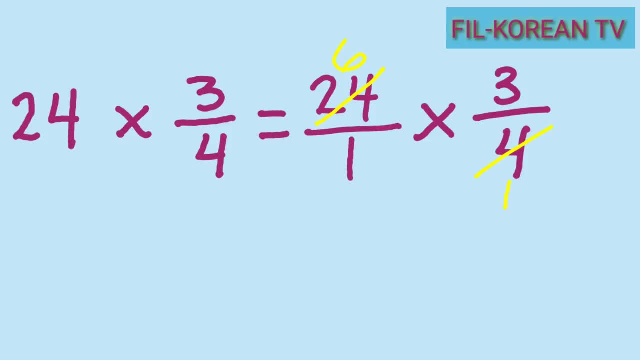 Kaya ang next step na gagawin natin ay imumultiply na natin yung numerators at saka imumultiply din yung denominators. Okay, so let's answer: 6 times 3 equals 18.. 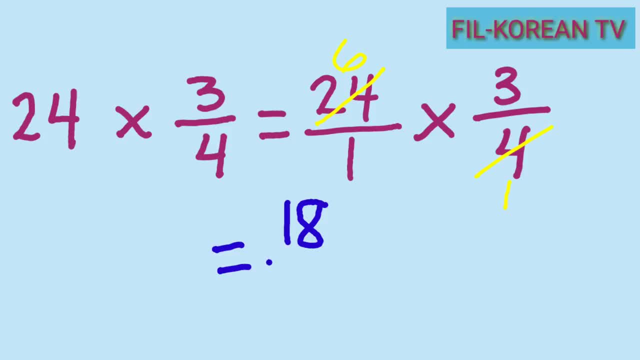 And 1 times 1 equals 1.. Okay, the answer is 18 over 1.. Improper fraction ito. kaya kailangan natin i-simplify, I-de-divide natin yung numerator na 18 sa denominator na 1.. 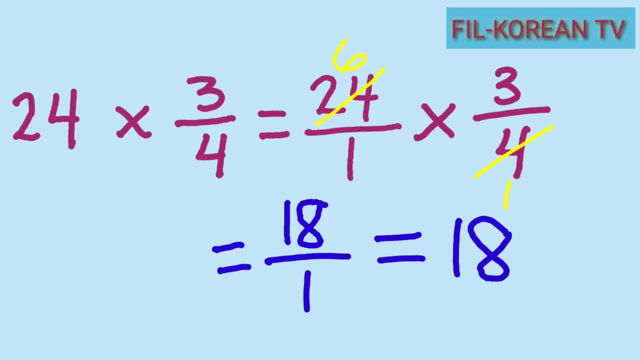 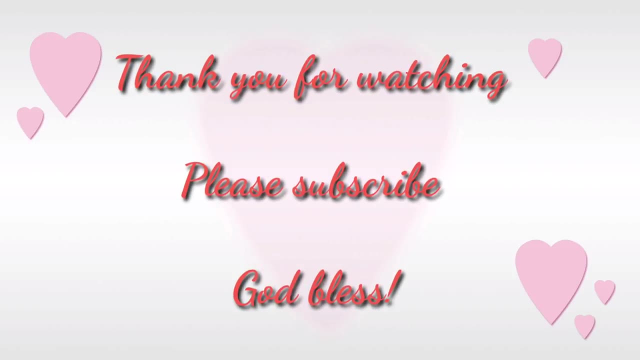 18 divided by 1, the answer is 18.. So the final answer is 18.. That's all for this topic. I hope you learned from it. See you next time, God bless. God bless.